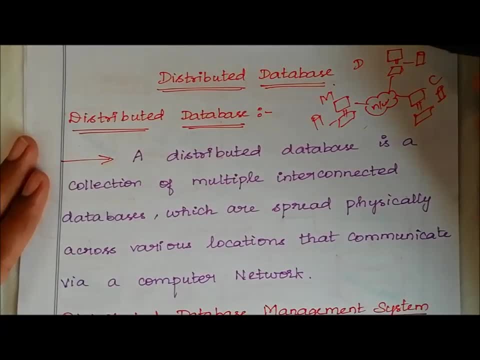 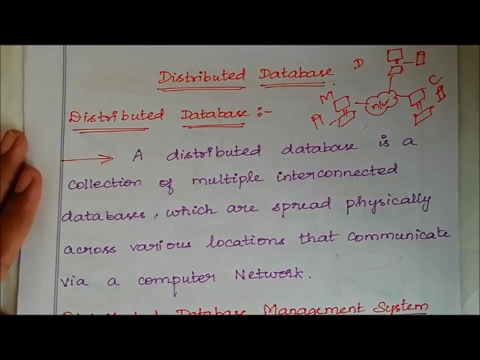 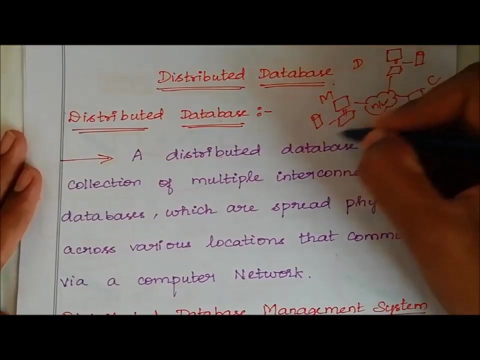 I am maintaining a database in chennai. I am doing everything by interconnecting by means of internet, so this is nothing but a distributed database. so a distributed database is a collection of multiple interconnected databases. so these are the databases, these are the databases connected with each system. 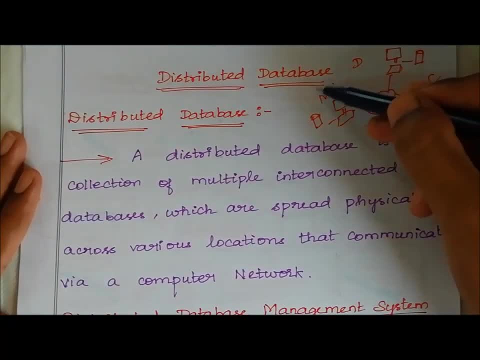 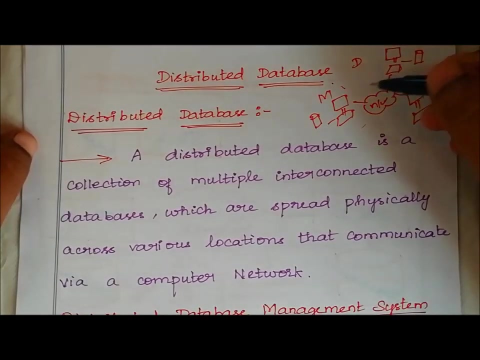 so here, for example, mobile users will access this database, chennai local users will access this database, just like a server. what is a server? I have kept it in different locations to be helpful to the user, to give a speedy response, but all the databases are connected to the network. 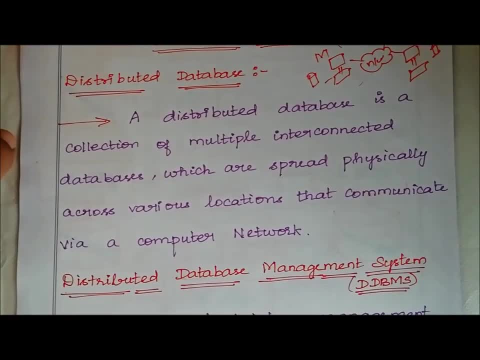 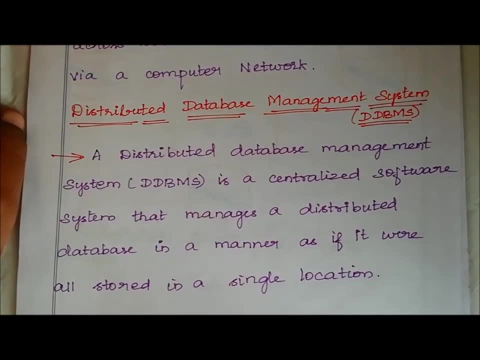 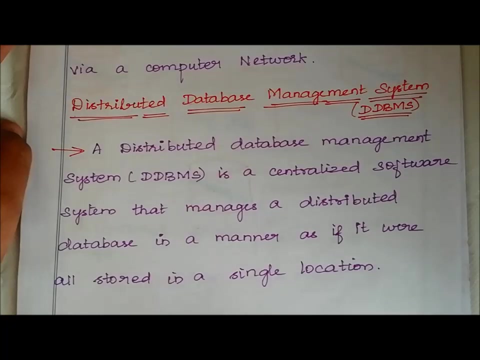 so this is nothing but a distributed database. so let's see what is a distributed database management system. a distributed database management system, that is ddbms, is a centralized server system that manages a distributed database in a manner, as it were, all stored in a single location. 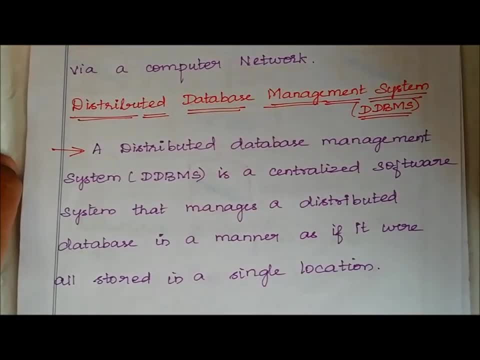 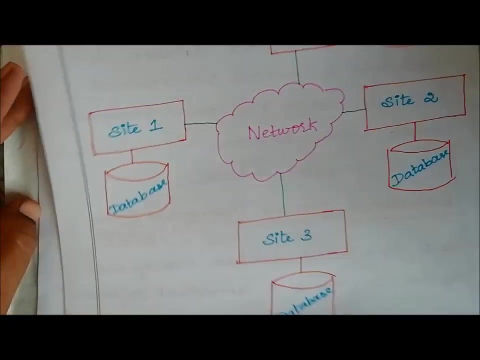 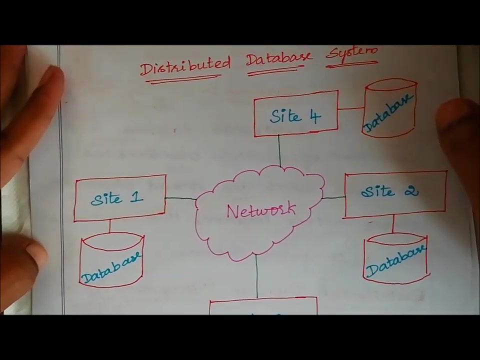 so that is distributed database, that is managing and controlling ddbms, that is distributed database management system. distributed database overall is controlled and managed. so let's see the architecture diagram of a distributed database system. consider the sites. sites is a system that is computer and distributor system. 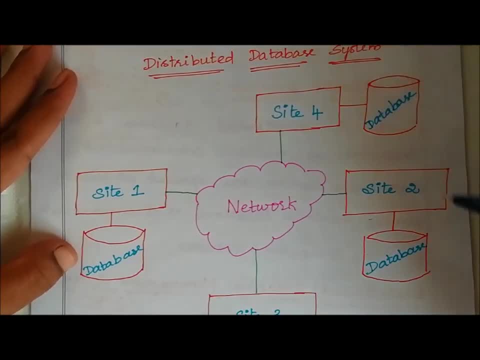 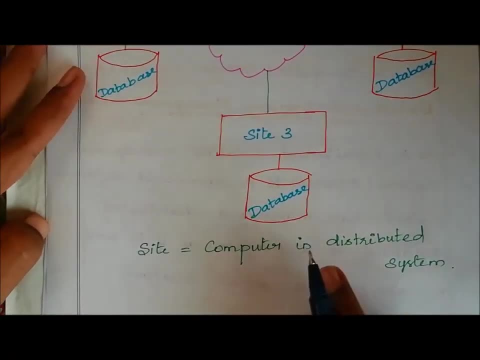 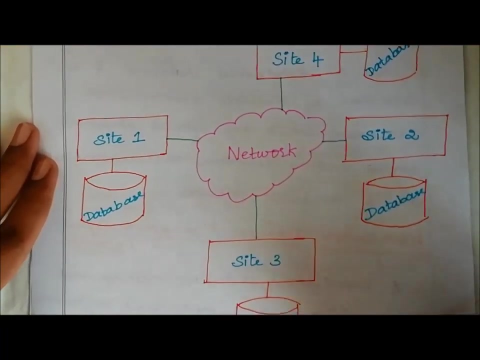 I have connected a database in site 4, as well as a database connected in site 2, a database connected in site 1, as well as a database connected in site 3. site is nothing but a computer and distributor system in which are PC as well as site. 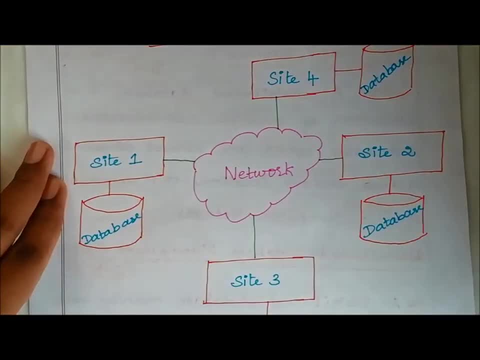 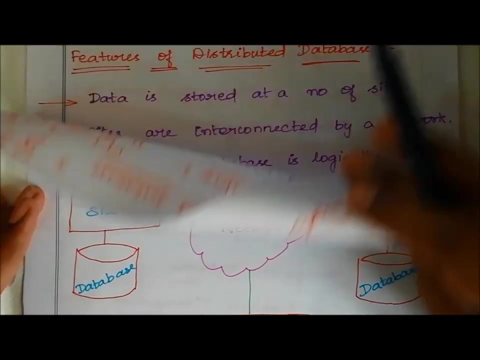 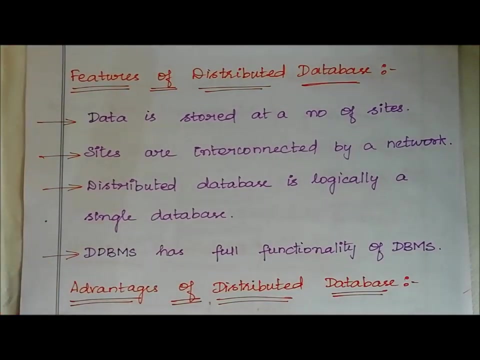 so all other sites will be connected by means of the internet connection. so through internet I have connected all the sites. these spatial connections spread over different locations by the network connection already used in computer. so this is the architecture diagram of distributed database system. So let's see the features of distributed database. So data is stored at a number of sites. So over sites we can easily access the location of the user. 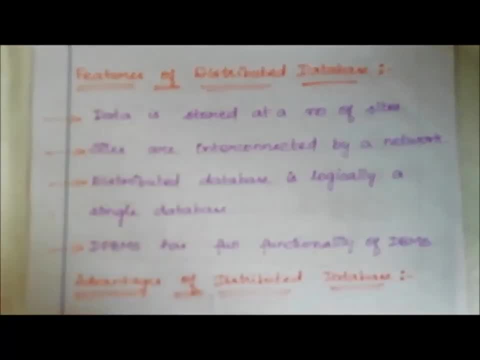 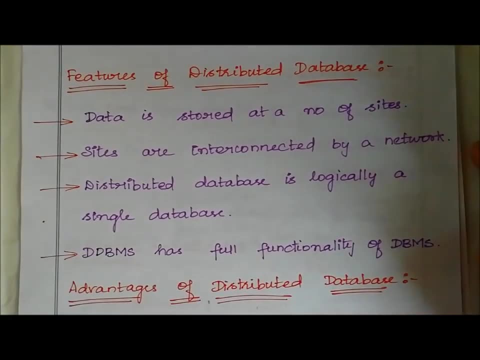 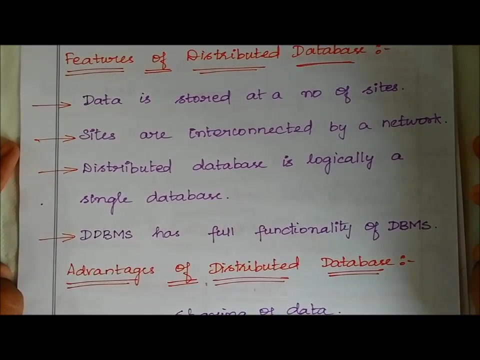 And also if the data was lost in some other location, then we can retrieve the data for our use. here Sites are interconnected by network, So each site would be that it be connected by means of internet. on an internet, normal And distributed database is logically single database. even then database would be displayed at different locations. 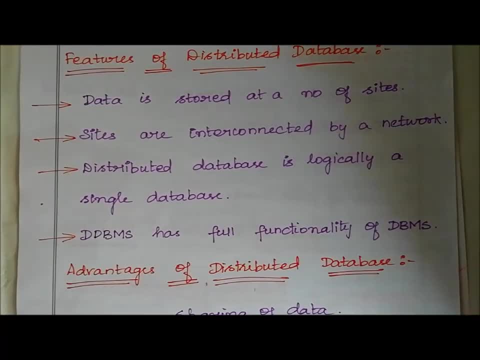 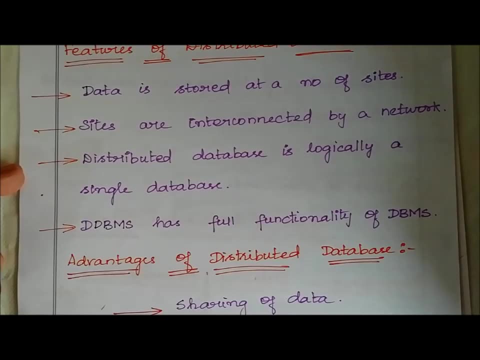 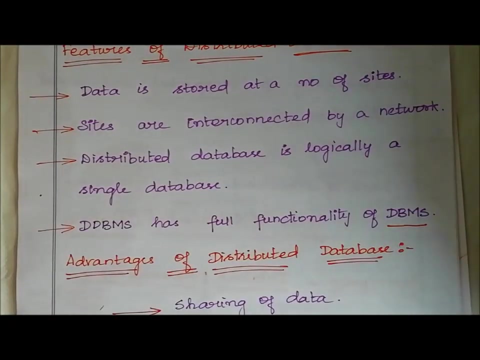 mayın, all databases will be considered as a single database, okay, and then that is distributed DBMS has full functionality of DBMS, okay. so if you are a DBMS executed, okay, that is database management system executed. the same functionality will be there. that is distributed DBMS. 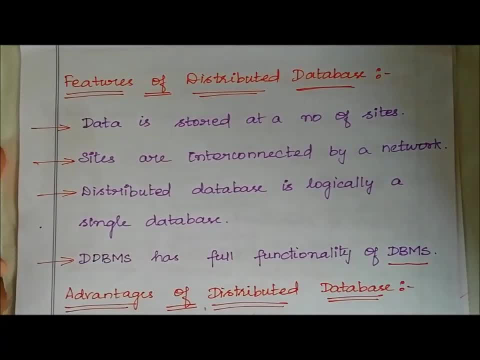 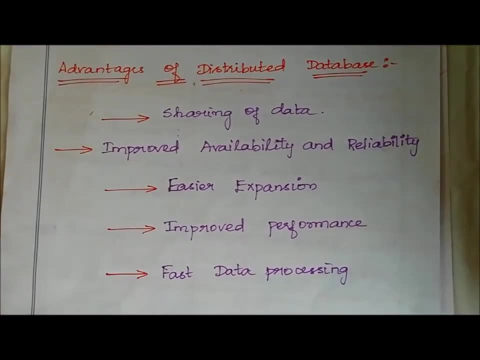 okay, so these are the some of the features of a distributed database. okay, let's see the advantages of a distributed database. sharing of data: okay. so on, the starting of data is possible in the distributed database because multiple locations where so anyone can access the data Thinking of. 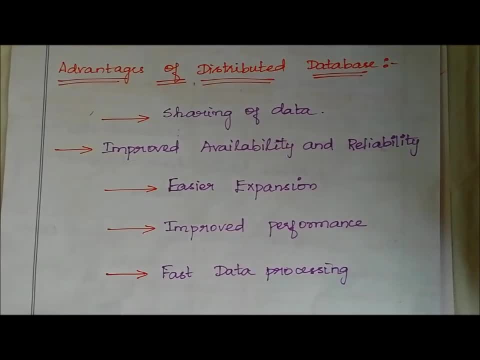 data is possible in distributed database. second one is improved availability and reliability. okay, so available, available. the Nara users can upon no headed to easier response. credit of Nara, your clients on the request, family response from the immediate response room because over location you may not believe, current over database with you. so immediate response I'll link on.